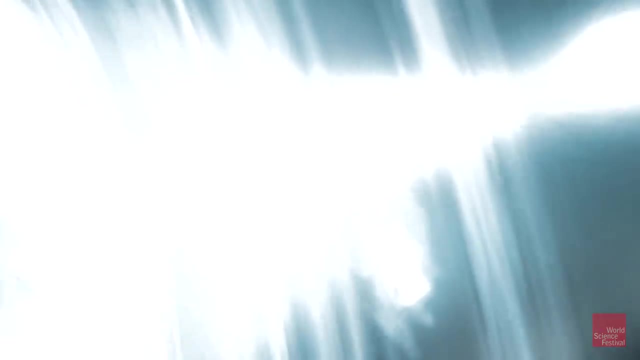 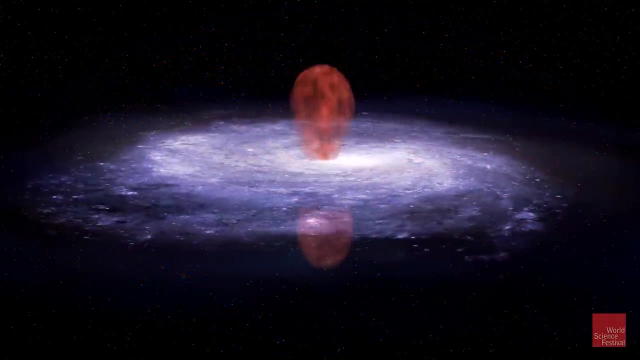 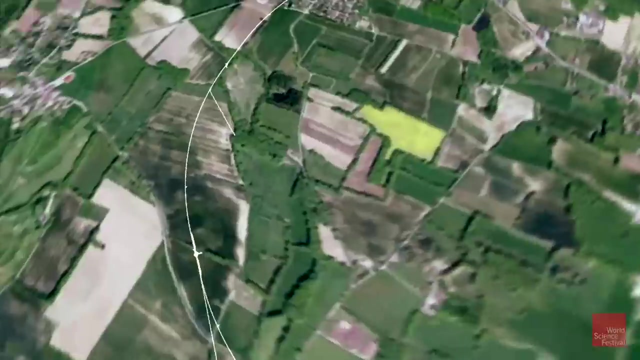 might produce things we can't see. That's what these satellites can detect, like gamma rays. The Fermi satellite has measured an excess coming from the direction of the center of our galaxy that may be caused by dark matter Back on Earth, rather than waiting for dark matter particles to arrive from space. there's 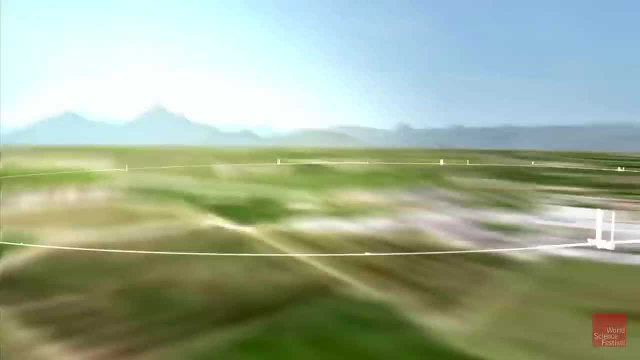 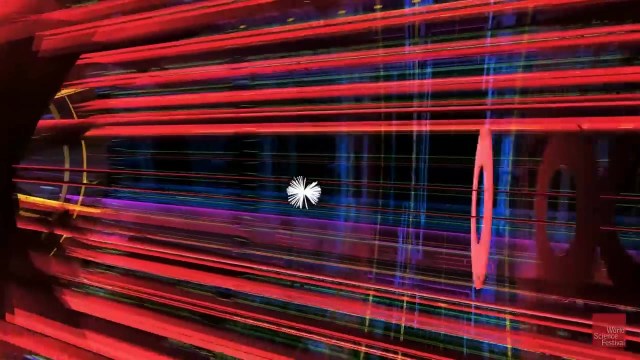 an experiment attempting to generate wimps from scratch by slamming protons together at nearly the speed of light. The violent head-on collisions convert this energy into showers of exoplanet energy. The light is then reflected by the light and the photons are then poured into the. 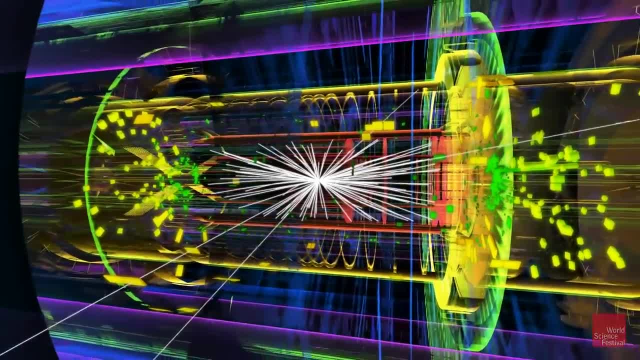 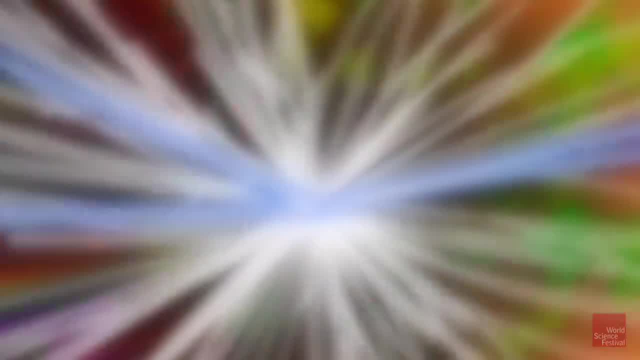 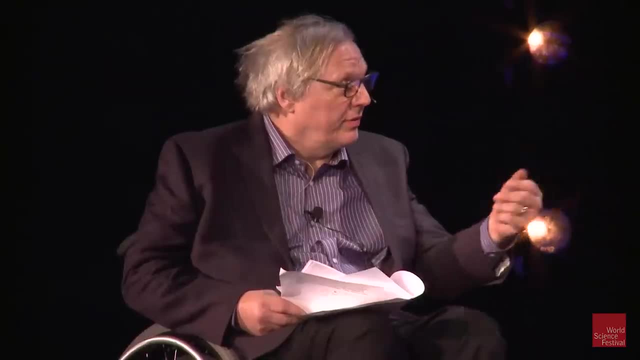 Towers of exotic particles scattering in all directions. Perhaps, within this debris, a short-lived dark matter particle will wink into existence. Do you go along with all those? by the way, That's a great video. I was going to talk about the three ways to detect it. There they are. 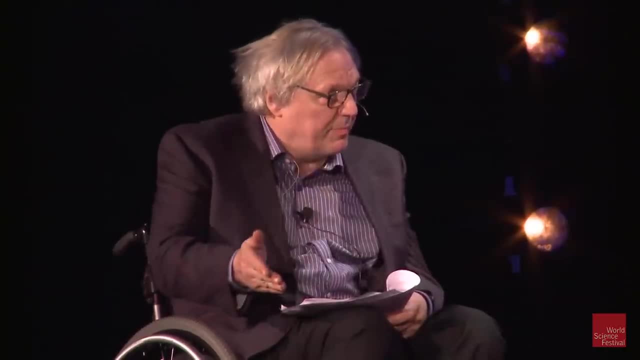 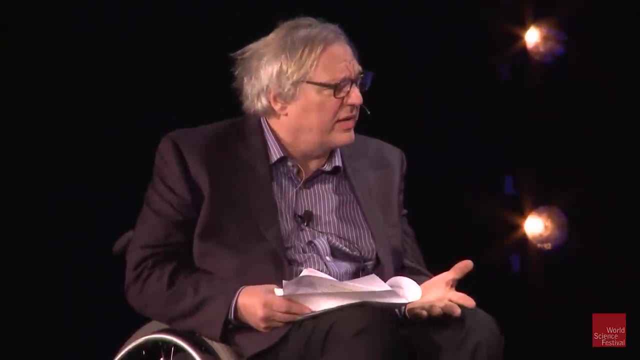 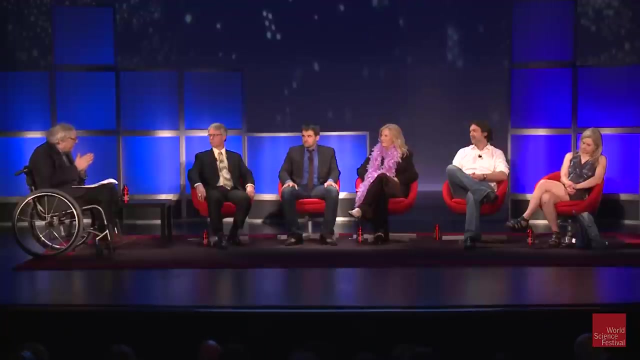 There they are. Well, is the first option, the deep in the mountains, deep in the mines, very quiet, isolating something away from all other forces? Is that something like the LIGO experiment to detect gravity waves, where you've got something on Earth that's trying to detect something that's very, very difficult to detect? 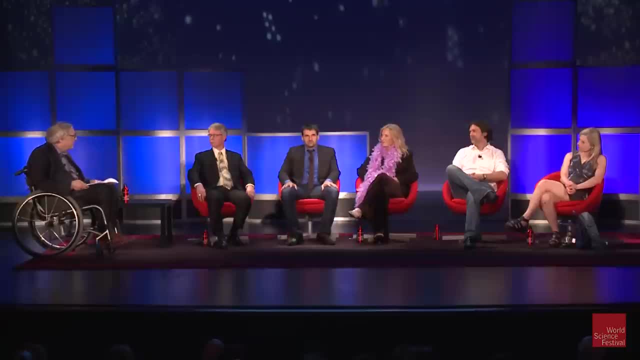 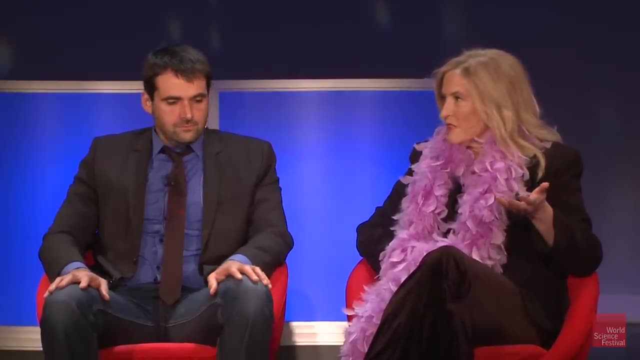 very, very sensitive and so this crazy kind of detector will, I mean because that was successful. Well yeah, these experiments, they are very difficult. So the count rate is: if you have a kilogram of detector, then you're going to get. 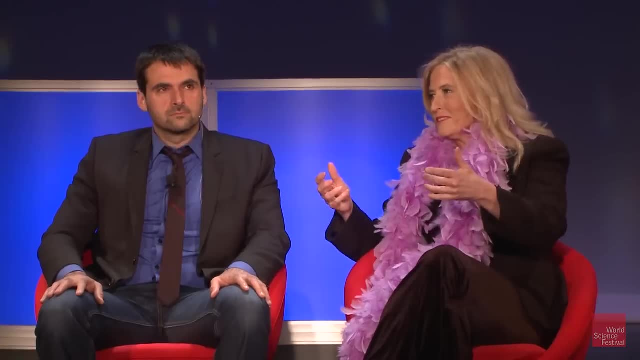 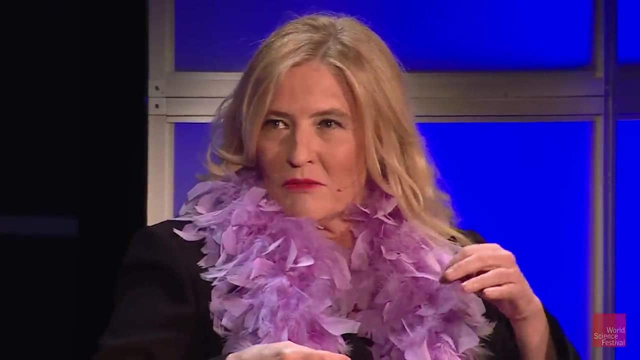 In a day, you might hope for one hit from one of these things, and you have to get rid of all the competing signals that there's a lot more of, And then the amount of energy that's deposited when there is a hit is really, really tiny. 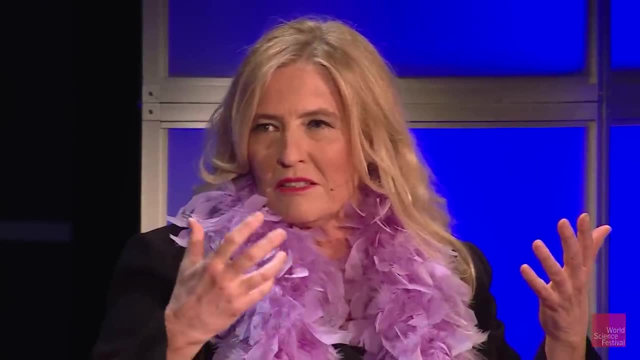 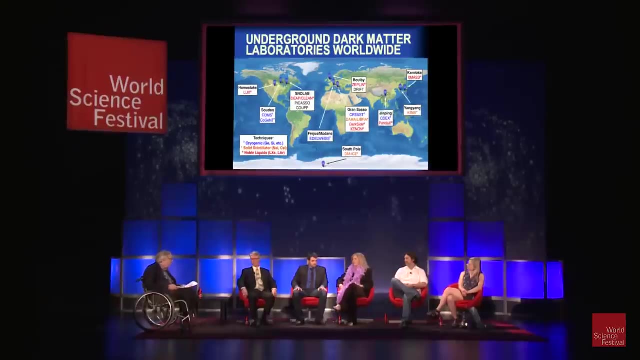 So you have to be really clever to find that this event ever took place. So, yeah, it requires really great sensitivity. So these experimentalists are awesome. So where do we stand in terms of, I mean, are they waiting? Are they still designing the software? Are the detectors sort of being? 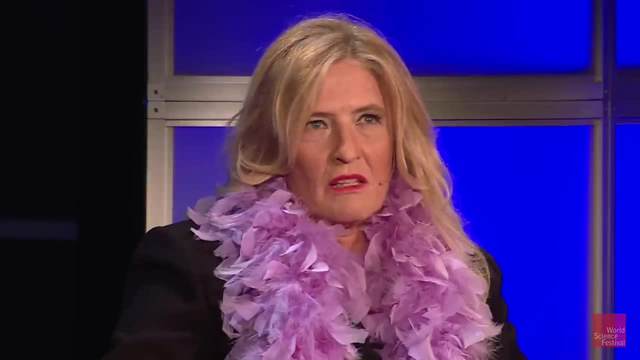 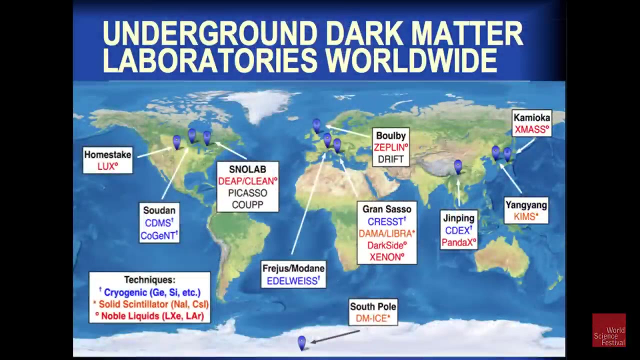 There's the slide shows that in the last 25 years there's been an explosion of these detectors and that's where they are. So they're all over the world and all the different continents, including underneath the ice at the South Pole.